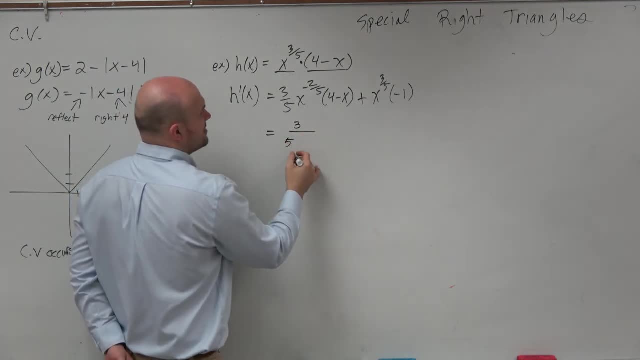 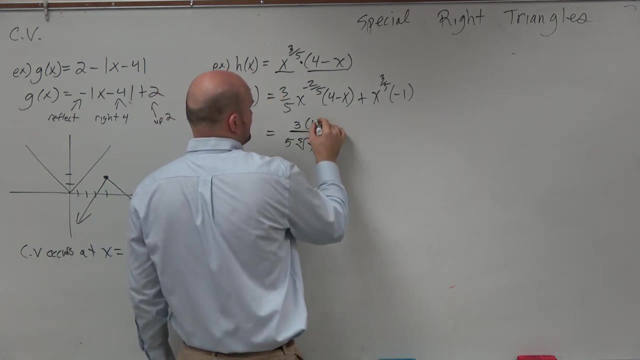 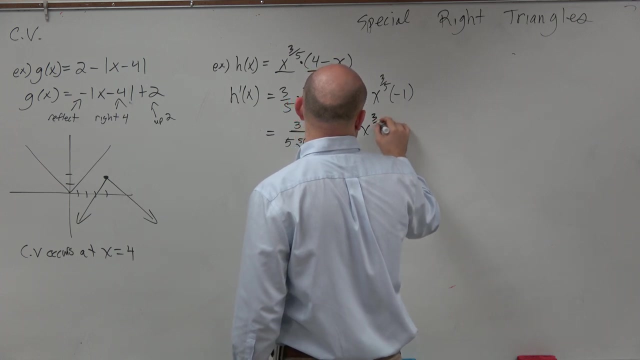 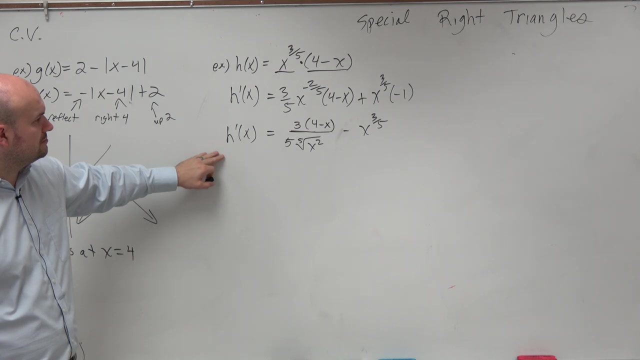 So we could have 3 over 5 times the fifth root of x squared, And that's going to be times 4 minus x, minus x to the 3 fifths. OK, well, so let's. so if we look at this guys, 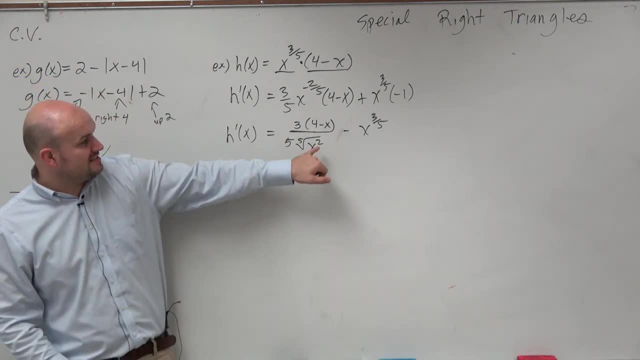 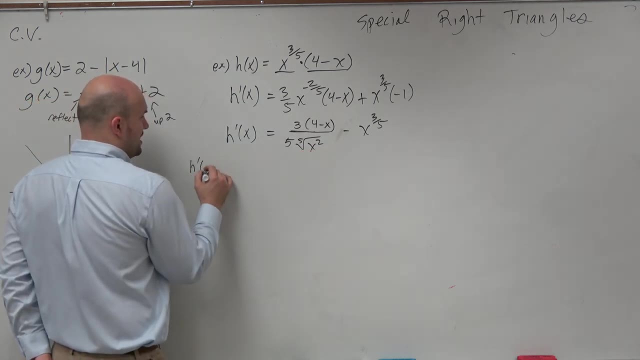 and we're just going to look at when this is undefined. wouldn't you guys agree? when x is undefined? Yes, Yes, So we could say that h prime of x is undefined at x equals 0.. Now we want to figure out when these are all equal to 0. 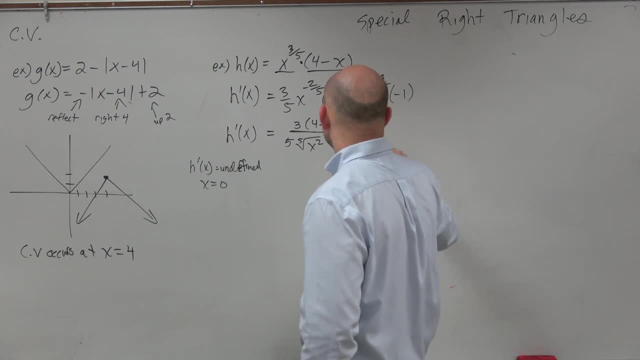 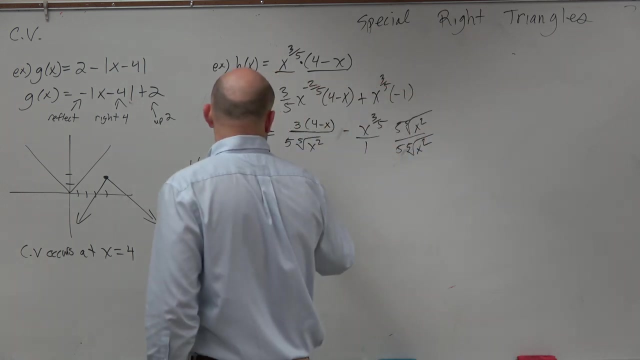 One thing I might want to do is actually combine these to get common denominators. So I can multiply by 5 fifth root squared of x squared, or 5 times the fifth root actually, Yeah, 5 fifth root of x? squared. so we'd. 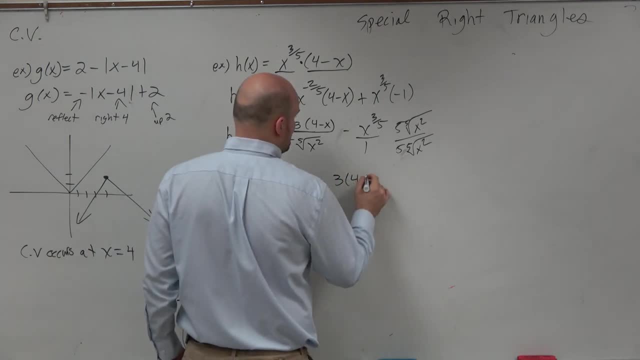 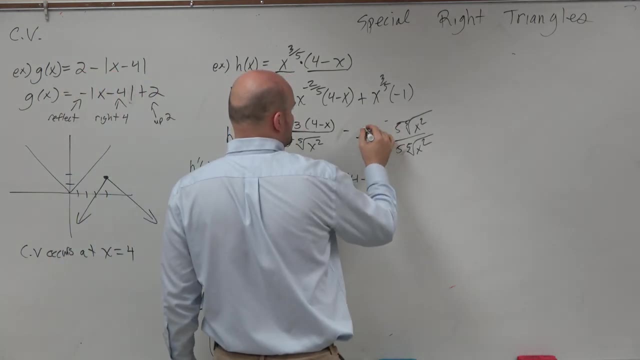 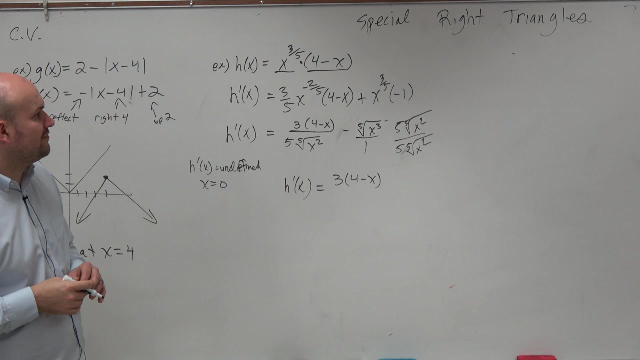 have h, prime of x is equal to 3 times 4 minus x times. let's see the fifth root of x cubed. Let's rewrite it like this: Fifth root of x cubed. so therefore that's going to be minus. you can multiply these. 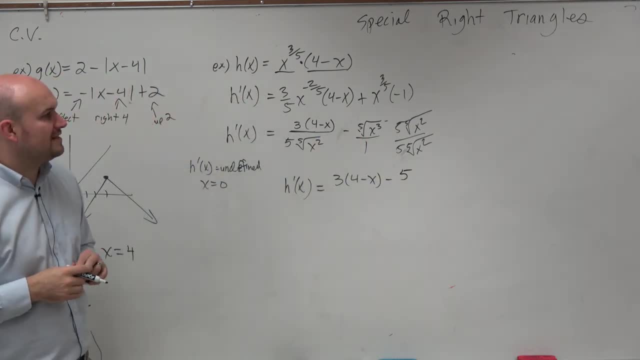 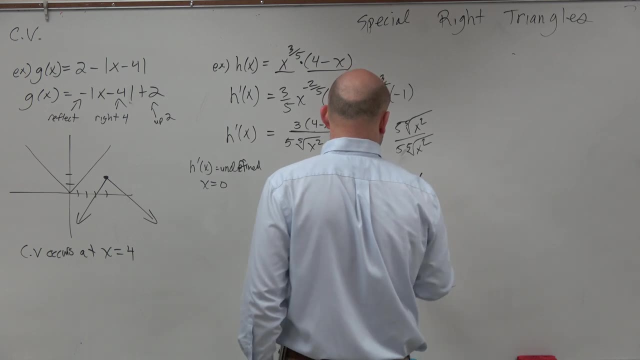 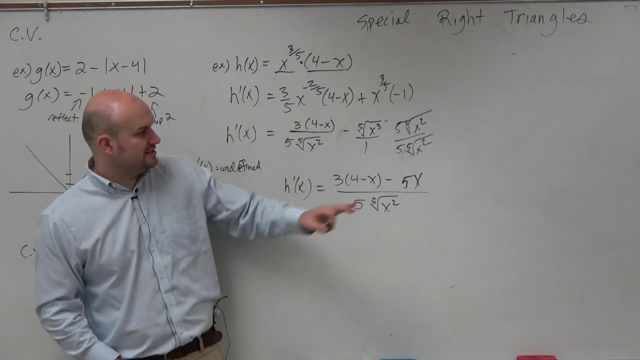 so that'd be 5. fifth root times x. cubed, you're going to add the power, so that's going to be the fifth root of x to the fifth, which is just going to be a 5x. Is anybody seeing where I just did some of that math? 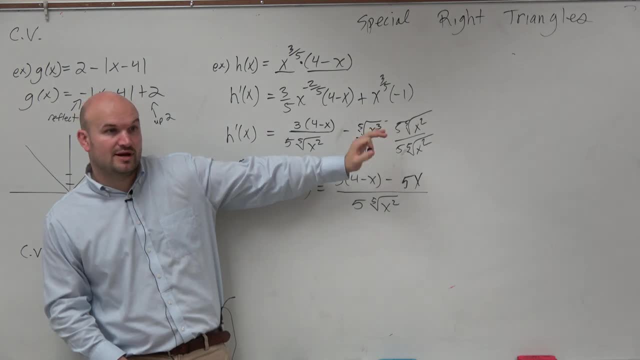 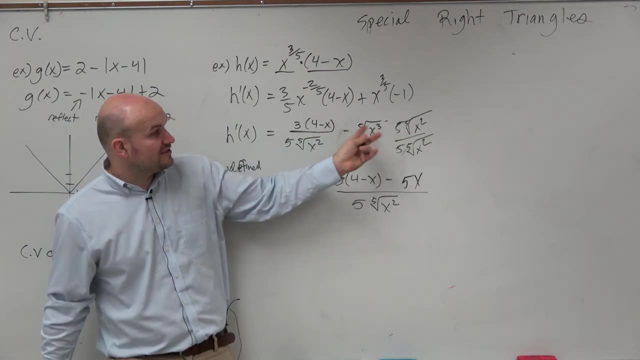 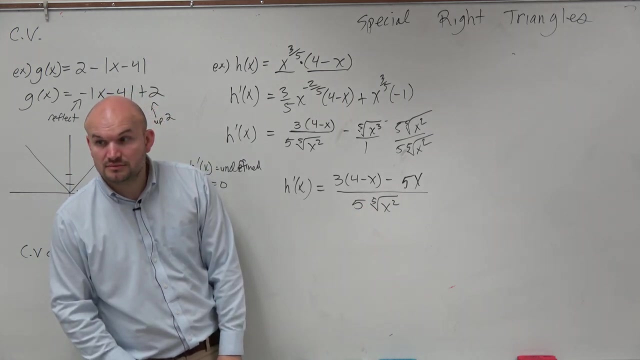 Does anybody see where I got it, or is everybody OK with that? If you're not, you can just say: hey, could you just? Is everybody OK with x cubed times? x squared is just x. No, Yes, no, maybe so.